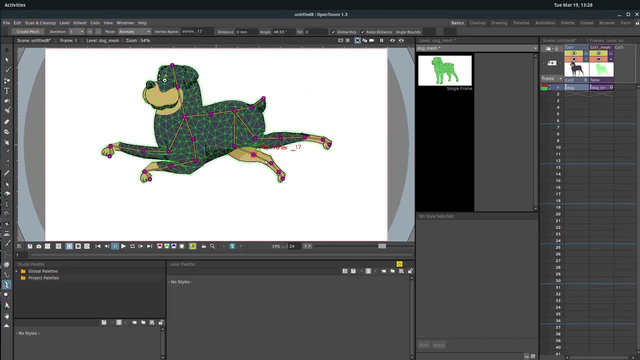 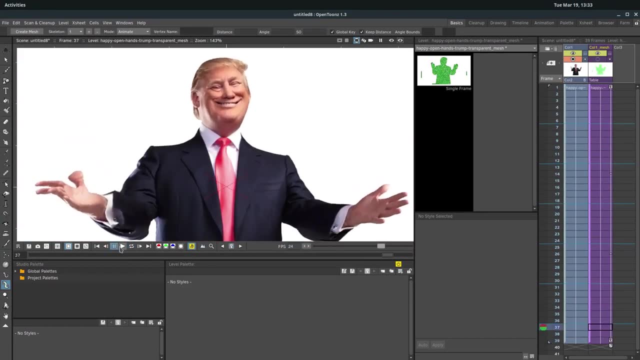 move that skeleton around to create either simple or advanced animations without having to redraw the image frame by frame every time. You can work with both vector and raster images, so bitmap and vector. It has a strong node based editor and you can interact with the 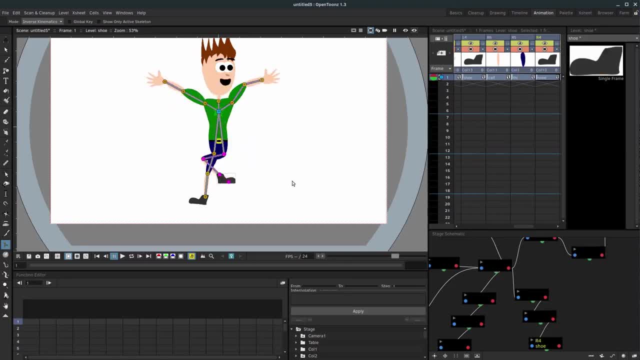 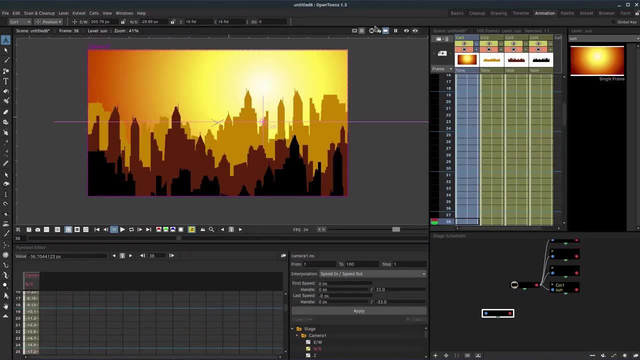 different effects. Here's the skeleton tool that's not using the mesh, So this is the one that's bringing in individual vector elements and then building a skeleton to them. You can set key frames. It has a really good X sheet and timeline. It's 2D but it does. 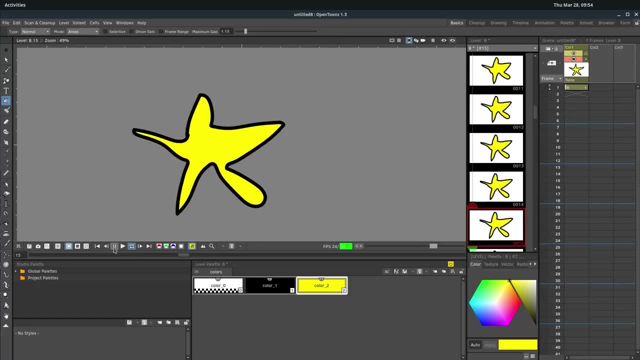 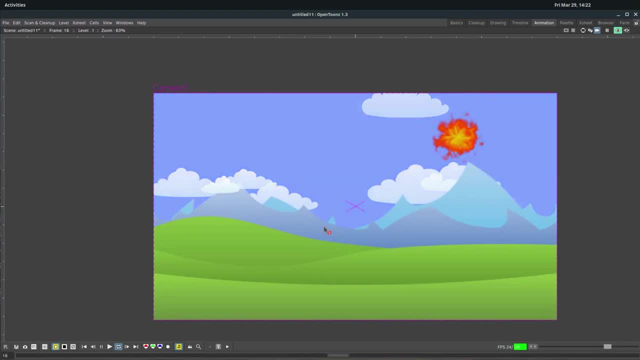 have a Z axis so you can work in 3D space somewhat. It's not completely 3D, Just a really cool tool. Go ahead and check out the links in the description to learn how to download this and get started using it, if it looks interesting to you. 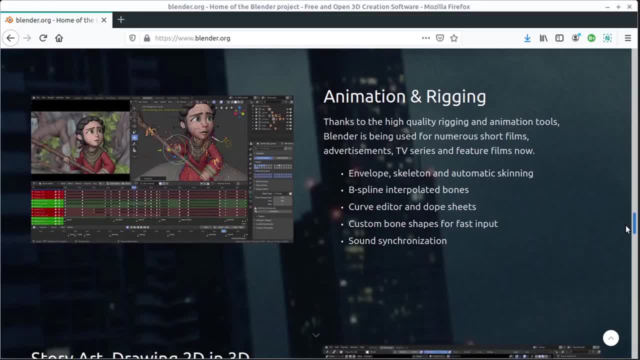 The next program we'll look at is Blender. Now, Blender is a 3D modeling program, but it does have a really good 2D model. It's a 3D model. It's a 3D model. It's a 3D model. 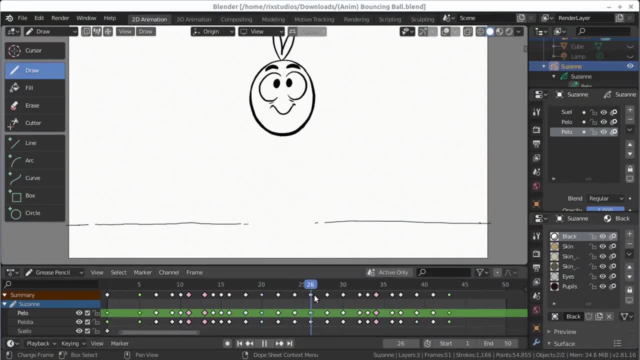 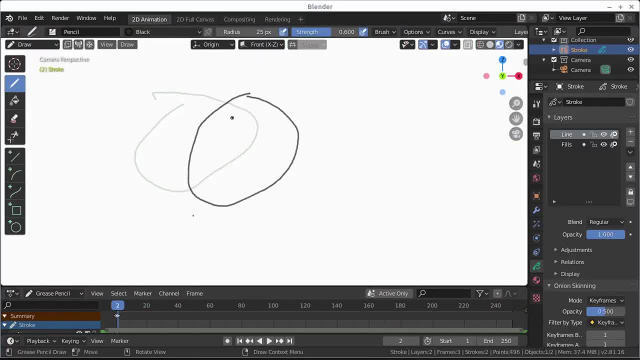 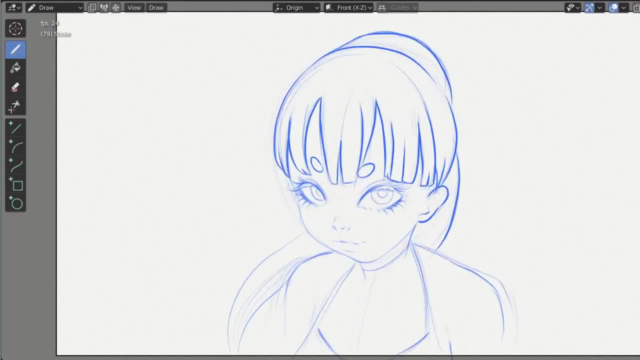 latest 2.8 release. They've really revamped the grease pencil and it has good drawing tools. Probably one of the strongest things for Blender is that it does have that true 3D space. Here's a time lapse of some drawing. Most of the things we're looking at here you 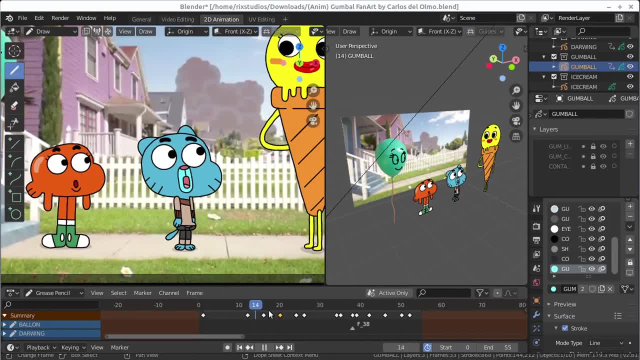 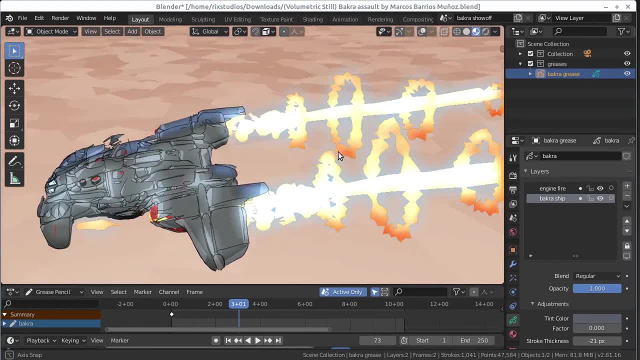 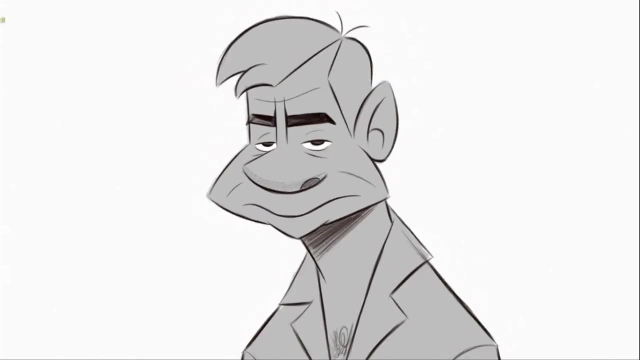 can actually download the source files. I just downloaded these from Blender and you can actually download them and see what's happening under the hood. There's a really large community of artists and creators and lots of good tutorials surrounding Blender. That's one of the huge, huge benefits of using Blender as a 2D animation tool. You can do frame-by-frame. 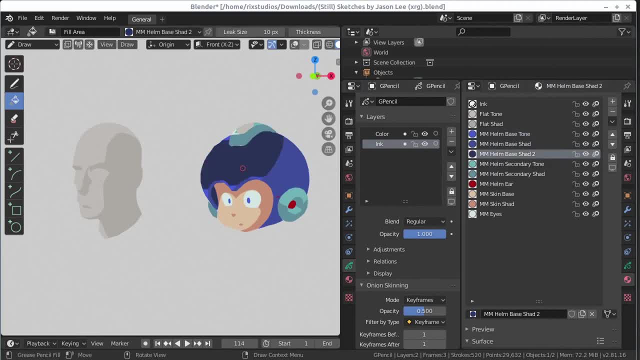 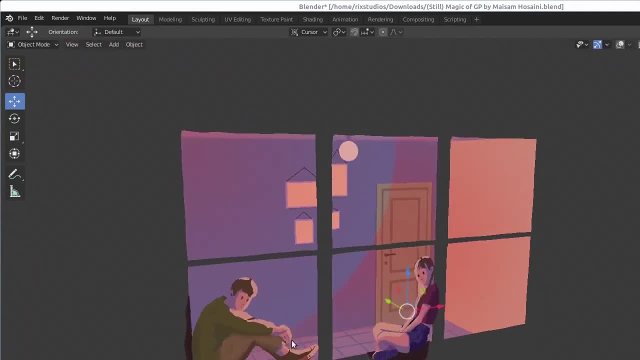 animation. You can have really good control over your different palettes and different materials and styles. Like I said, you can work in the 3D space really well to create some sort of 2D 3D looks, So a really good tool to look at if you're interested in 2D animation. 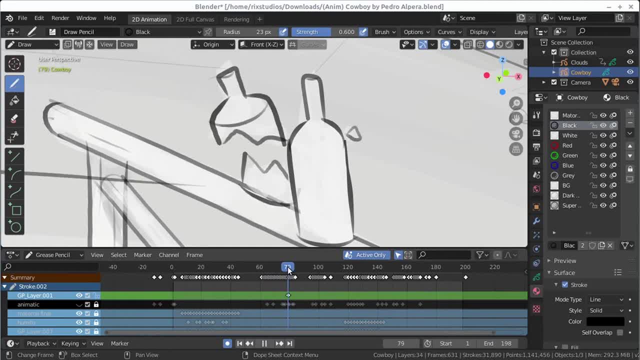 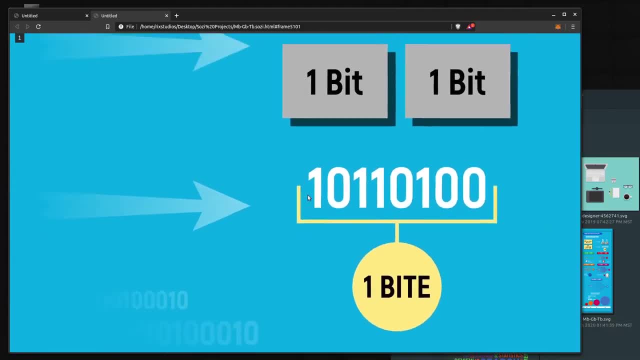 especially if you already have experience using Blender. This next program is Sozi. Sozi doesn't have any built-in drawing tools and it's more of a presentation tool, but it allows for vector animation and it's very basic and easy to use. So you create the artwork in something like: 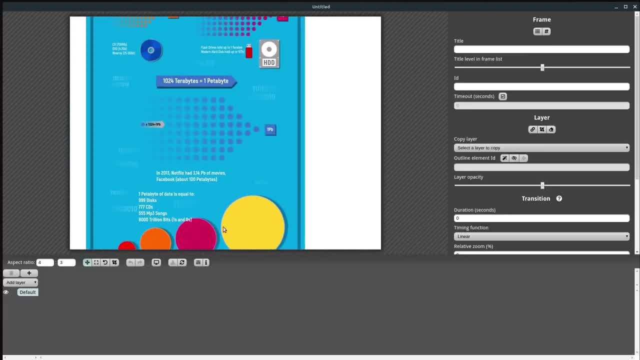 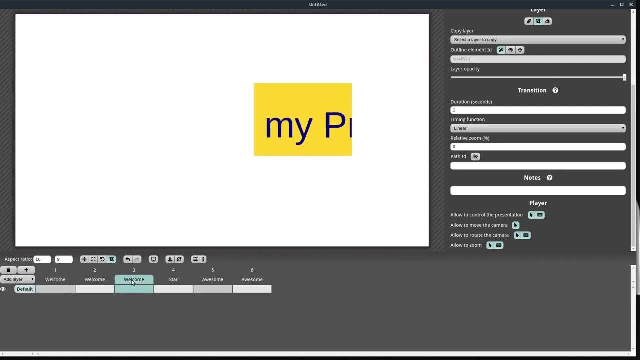 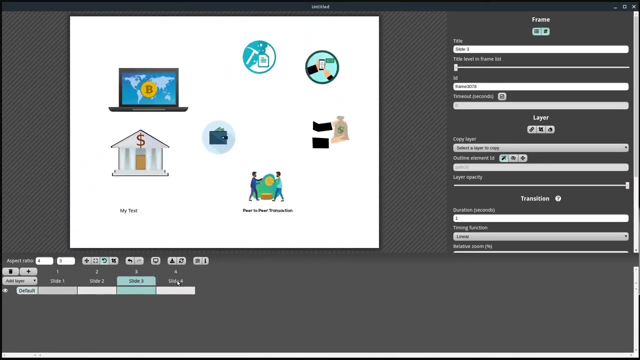 Inkscape. It accepts an SVG file and then you choose how the camera pans around and rotates and interacts and what part of the canvas you're able to see. You can also use this to create basic animations, because you can animate, you can control the position and location and the 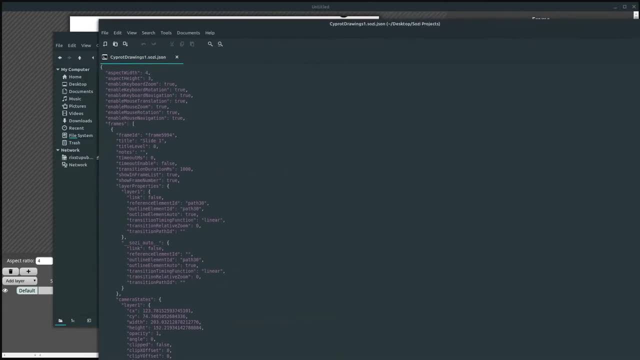 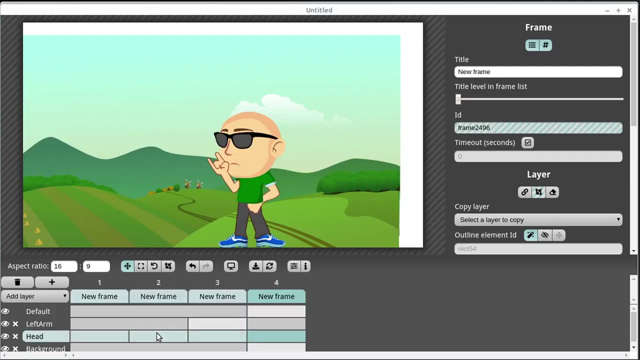 viewability or the visibility of each individual layer. One of the great things is it gives you all the code. It gives you the HTML and JSON file. You can embed this in a website. So if you want to create animations for the web, this might be a good tool to do, especially if you have 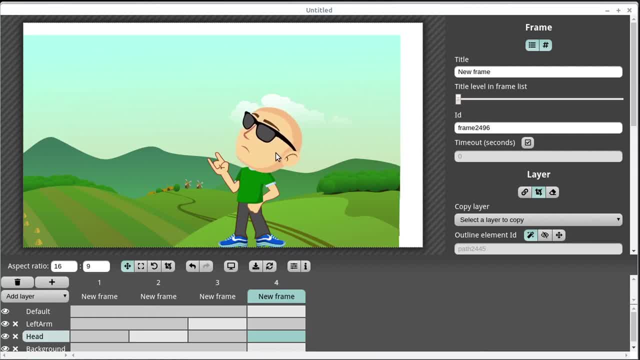 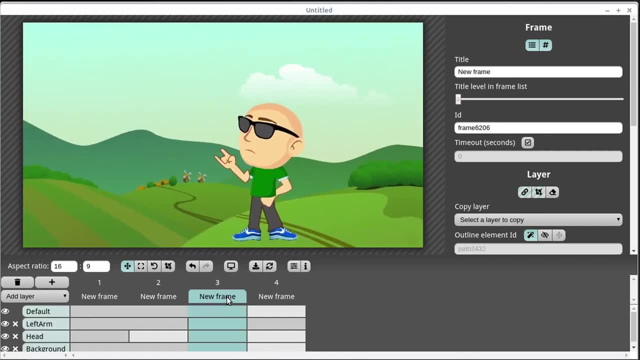 more of a programming web developer background. Like I said, it's a very basic tool. It's still under active development and it's a pretty small development team, But something to look into if you're interested in animating vector graphics, especially if you want to embed them in a 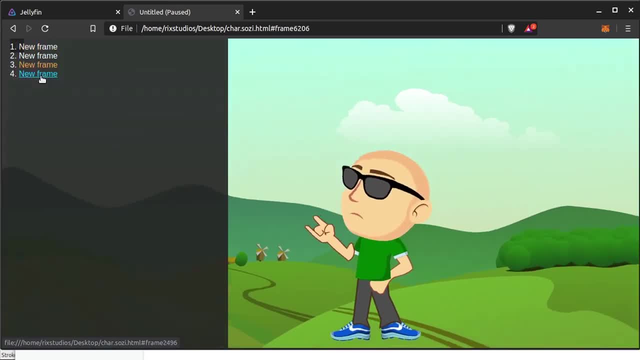 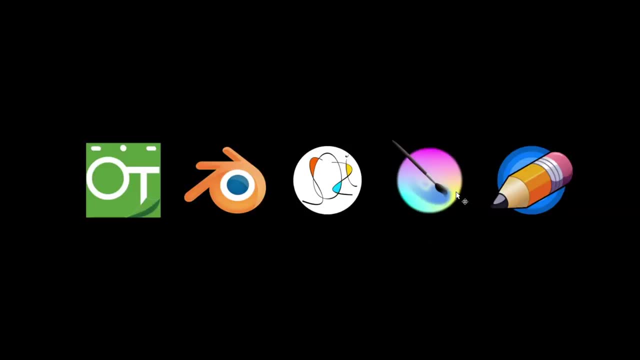 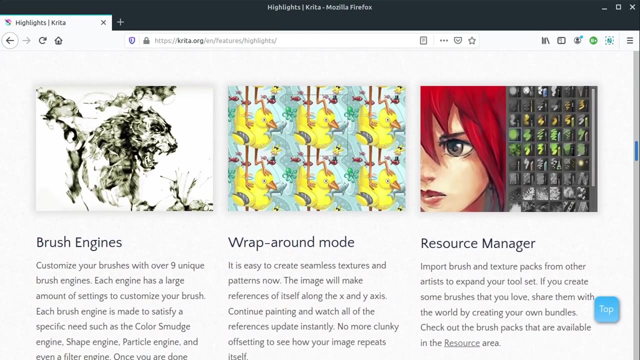 website. There is a third party plugin to export the final result in a video format as well. This next program is Krita. Krita is an outstanding program for creating digital art. It has great support for working with layers and different brushes and really just helps you recreate that. 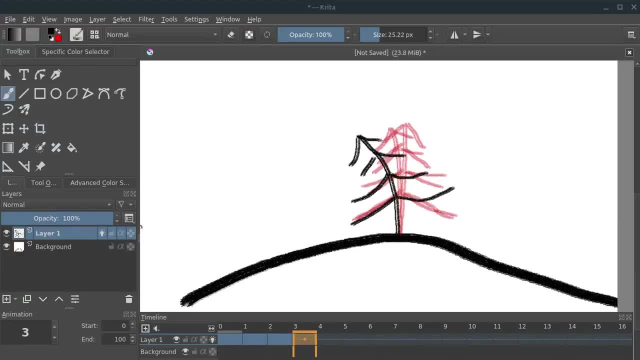 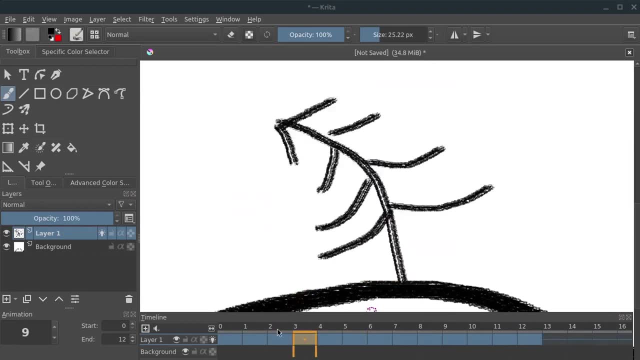 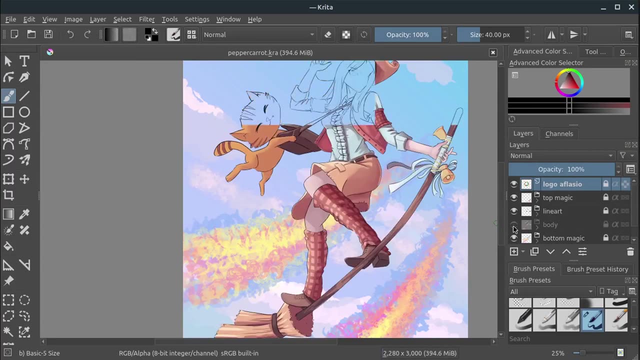 feeling of creating a traditional painting on a canvas, but in a digital format. It also has a lot of fun with the animation, So this timeline supports multiple layers. You have access to all the great art creation tools available in Krita, But the animation part is kind of a secondary. 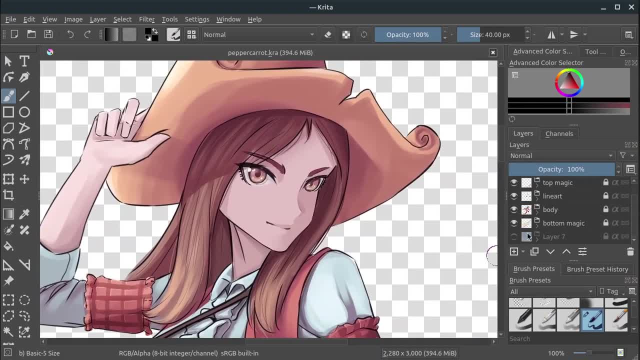 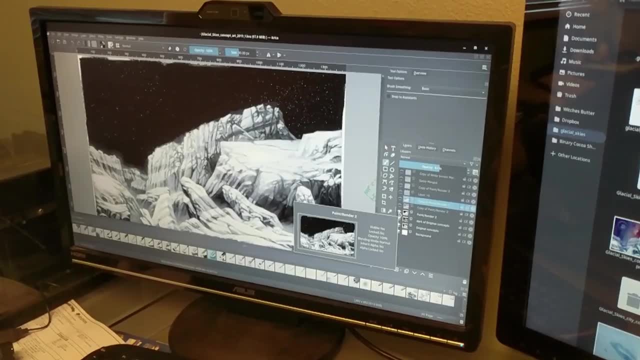 feature added in The primary focus is just creating art. People use this for comic books, People use it for all kinds of fan art creation and just any kind of art that you can imagine. Anything you could paint on a canvas you can paint digitally. This is very commonly used together. 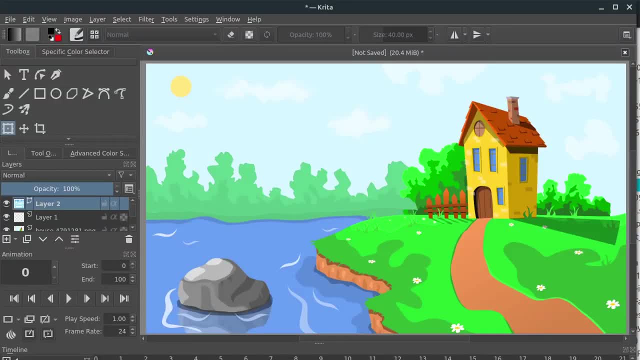 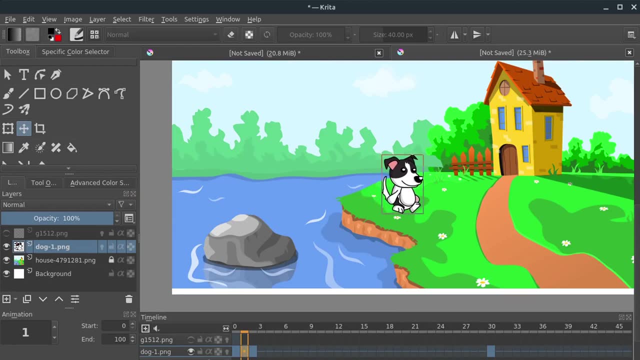 with a drawing tablet And it just has excellent, excellent support for drawing. You can bring in vector art, You can bring in raster or bitmap images And then you can keyframe those. You can change the camera, view what the camera can see, And so everything that we've seen. 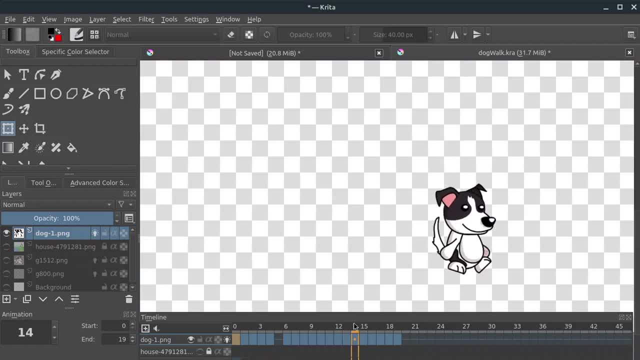 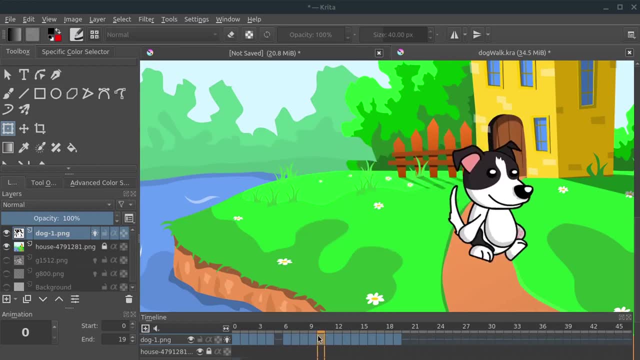 in these other programs. of course, Krita can do as well. It's a great tool to look into, especially if you're using a drawing tablet. Of all the ones in this list, this probably has the best support for creating art with a drawing tablet. This last program is Pencil 2D. Pencil 2D is a great program.